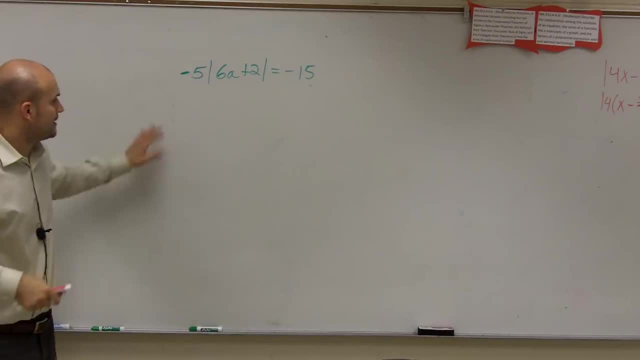 Okay, welcome. What I want to do is show you how to solve this absolute value inequality. So it's important that when you're solving absolute value inequalities, we need to make sure that we understand, first of all, our two cases, But before that, we need to understand how are we going to. 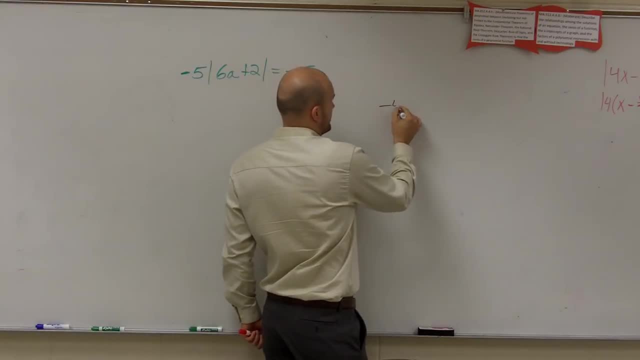 get to two cases. So let's go back and talk about absolute value inequality. Remember, absolute value. inequalities say the absolute distance from zero. So if I say the absolute distance, and that's talking about like on a number line- So if I have zero, one, two, three, four, 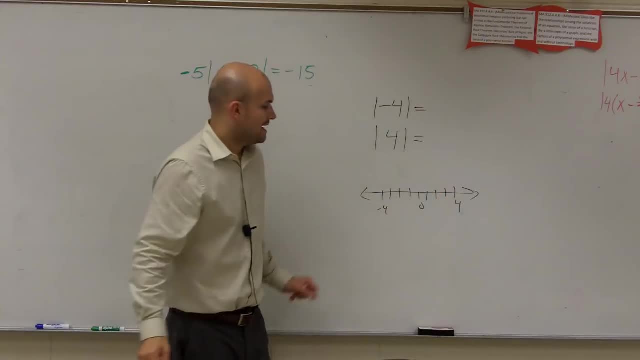 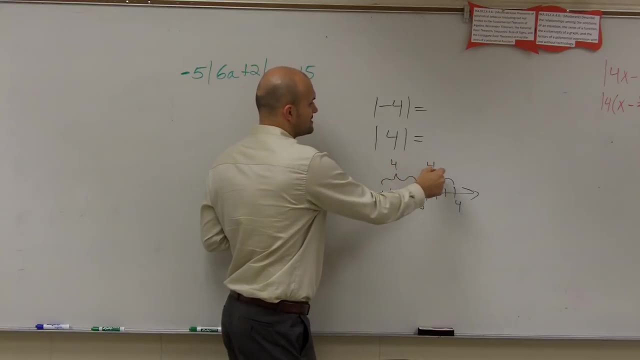 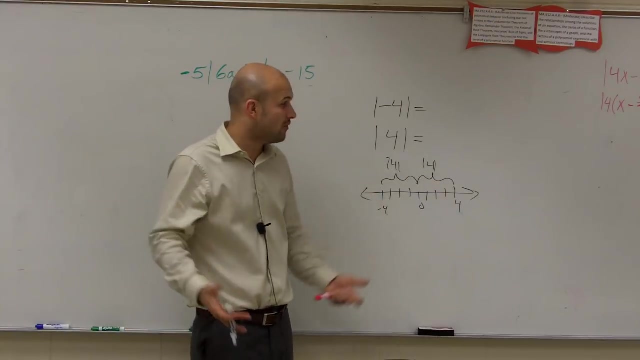 one, two, three, four, All right. And when I'm looking at the distance from negative four to zero and zero to four, I notice that both of those distances are what we call the absolute value. They, the distance you get from zero to negative four and from zero to four is both four. So 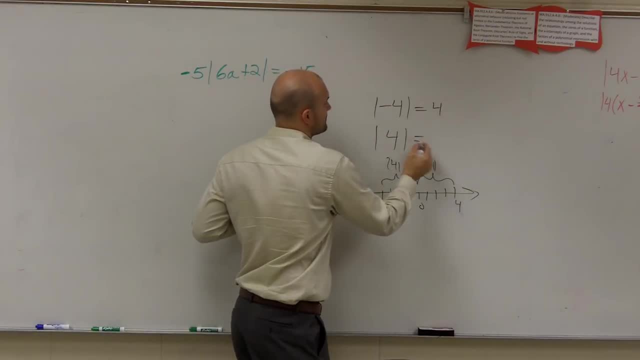 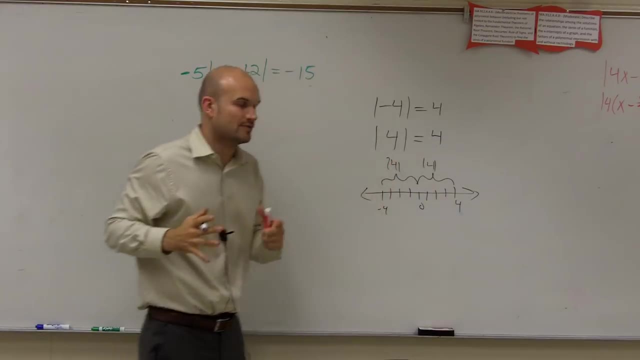 therefore, the absolute value- absolute value of negative 4- is equal to 4, and the absolute value of 4 is also equal to 4.. So the distance between both of these is what we call the absolute value 4.. So to do that, what we need, 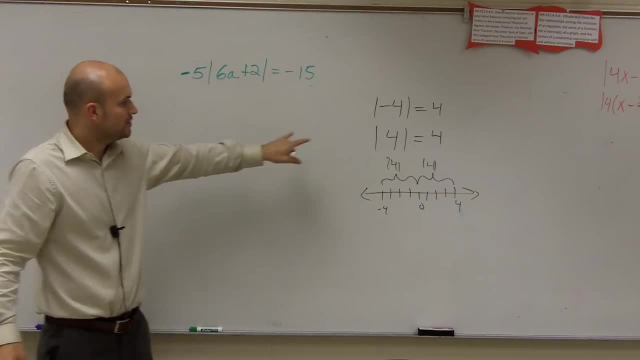 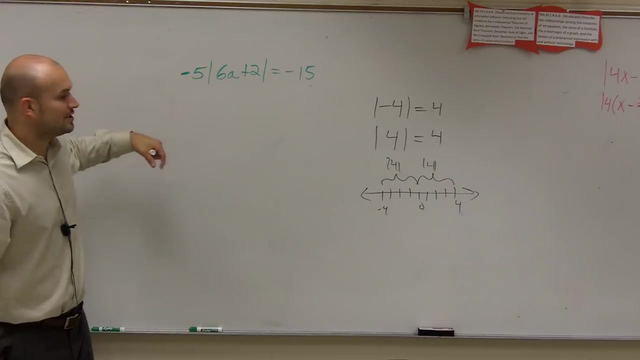 to look at here is: I need to get an absolute value by itself. Notice, my absolute value equals my number. So when I'm solving an absolute value, I need to first make sure I isolate my absolute value sign, meaning I get my absolute value sign all by itself. So I look at this and I'm going to 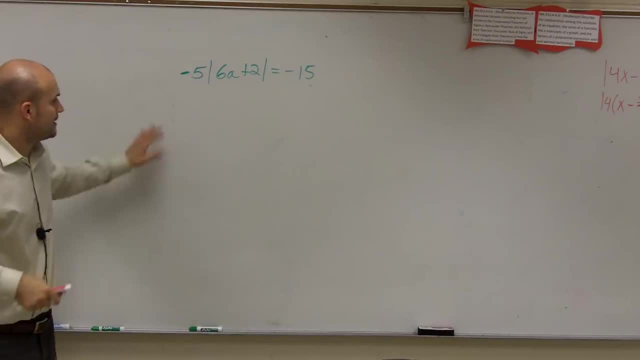 Okay, welcome. What I want to do is show you how to solve this absolute value inequality. So it's important that when you're solving absolute value inequalities, we need to make sure that we understand, first of all, our two cases, But before that, we need to understand how are we going to. 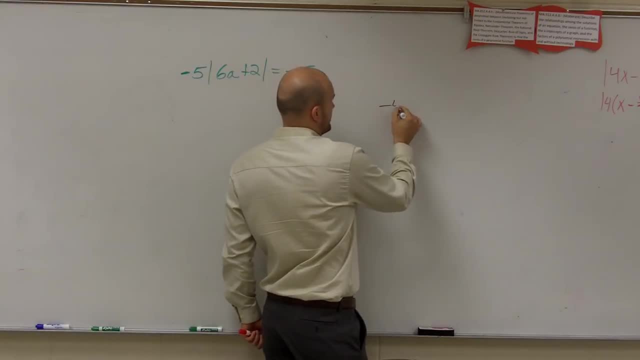 get to two cases. So let's go back and talk about absolute value inequality. Remember, absolute value inequality say the absolute distance from zero. So if I say the absolute distance, and that's talking about like on a number line, So if I have zero, one, two, three, four, 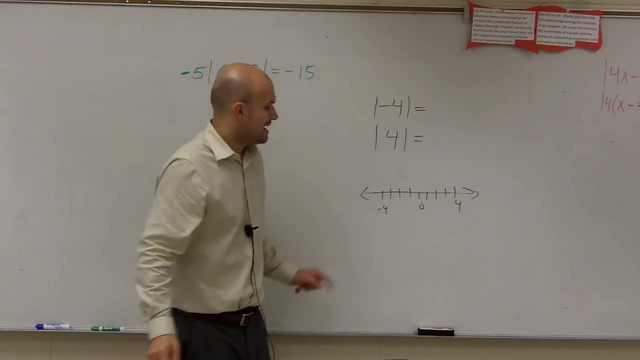 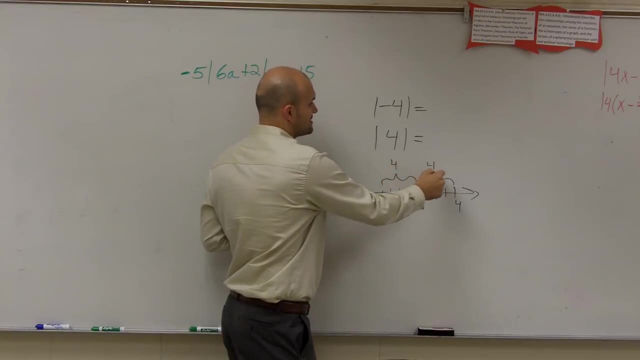 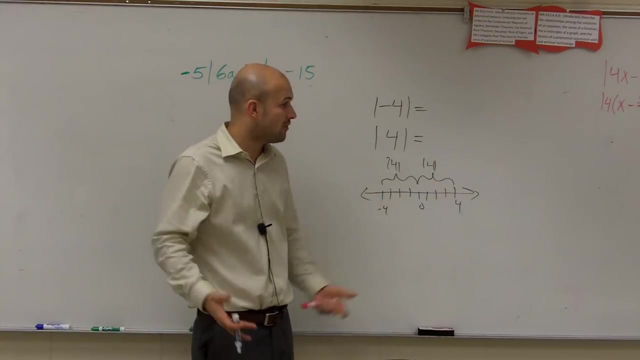 one, two, three, four, All right. And when I'm looking at the distance from negative four to zero and zero to four, I noticed that both of those distances are what we call the absolute value. The distance you get from zero to negative four and from zero to four is both four. So therefore, 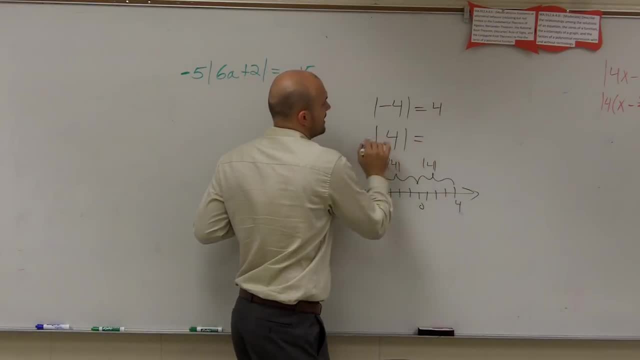 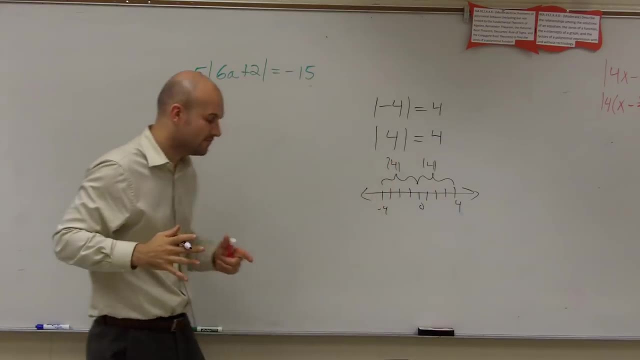 the absolute value. inequality is the absolute distance from zero to zero to four. So if I say absolute value of negative four is equal to four and the absolute value of four is also equal to four. So the distance between both of these is what we call the absolute value four. So 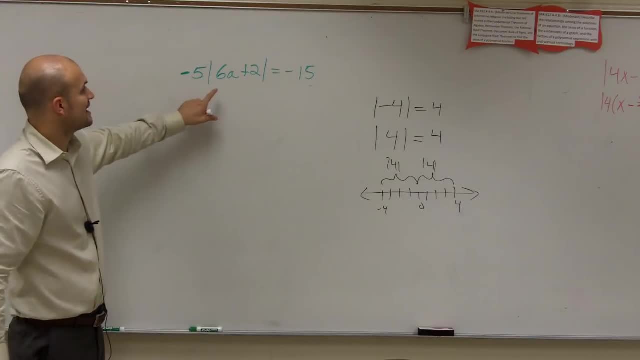 to do that. what we need to look at here is: I need to get an absolute value by itself. Notice: my absolute value equals my number. So when I'm solving an absolute value, I need to first make sure I isolate my absolute value sign, meaning I get my absolute value sign. 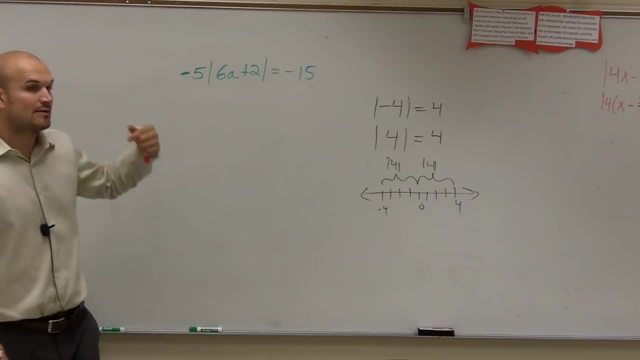 all by itself. So I look at this and I'm going to use my reverse order of operations to undo what's happening to my absolute value sign. And I look up here and I can say: all right, my absolute value sign is being multiplied by negative five, So I'm going to divide by negative. 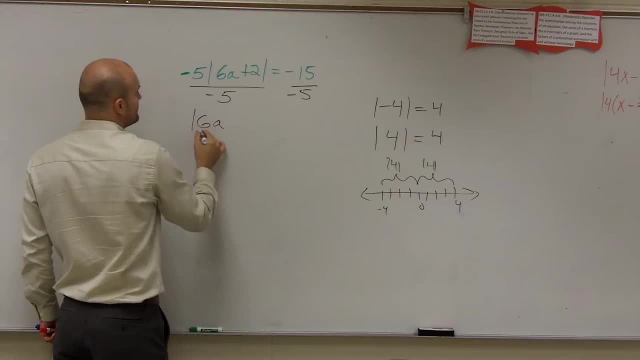 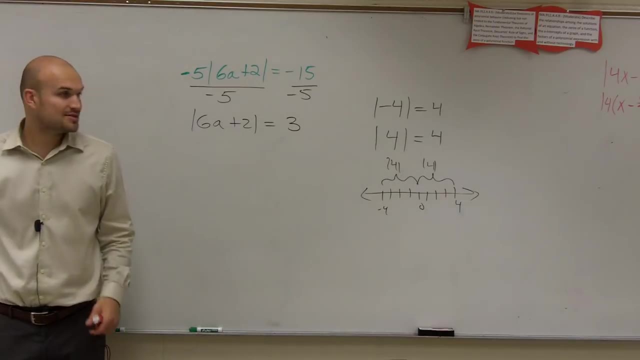 five. When doing that, I'm now left with absolute value of six. a plus two equals a positive three. All right, So now we come into the lovely case. All right, So what this states, if I was going to say this out loud, the absolute value of six times a number. 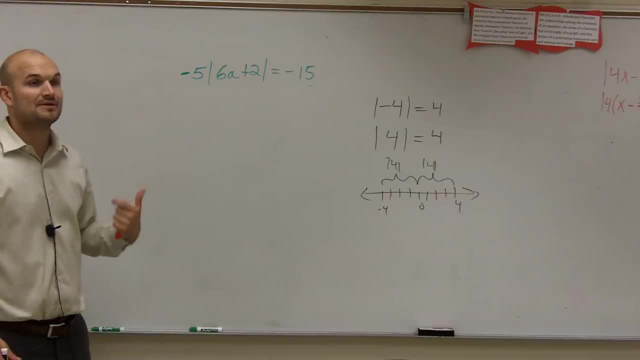 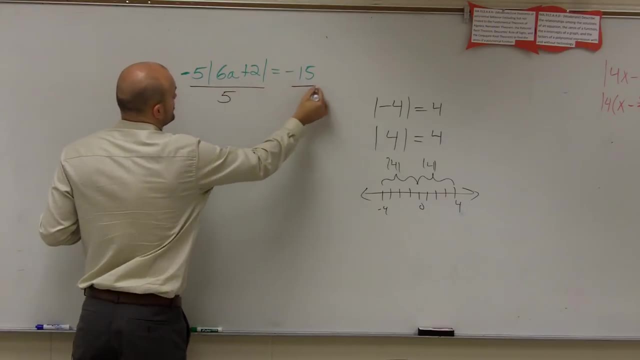 use my reverse order of operations to undo what's happening to my absolute value sign, And I look up here and I can say: all right, my absolute value sign is being multiplied by negative 5.. So I'm going to divide by negative 5.. When doing that, I'm now left with absolute value of 6a plus 2 equals. 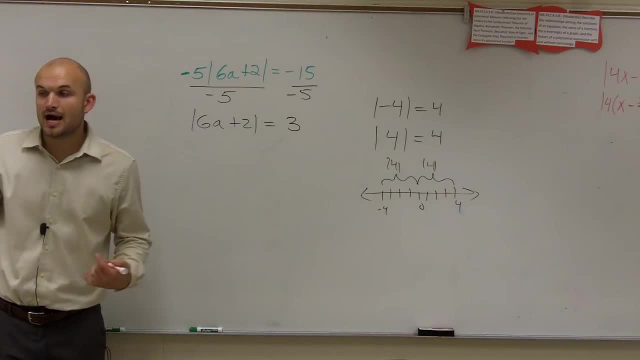 a positive 3.. All right, so now we come into the lovely case. All right, so what this states? if I was going to say this out loud, the absolute value of 6 times a number plus 2 is equal to 3.. Now remember for it to equal 3, we could have inside of here, could? 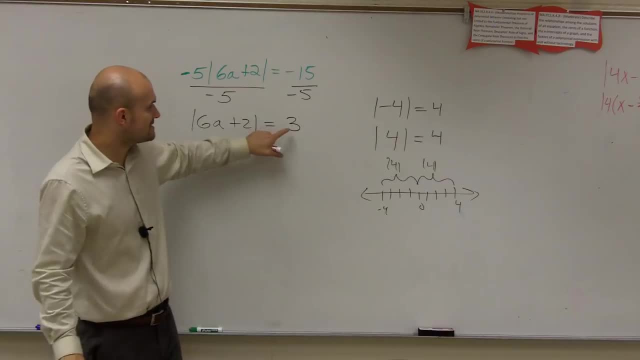 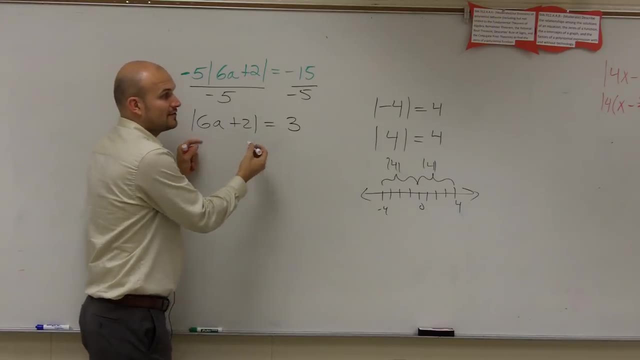 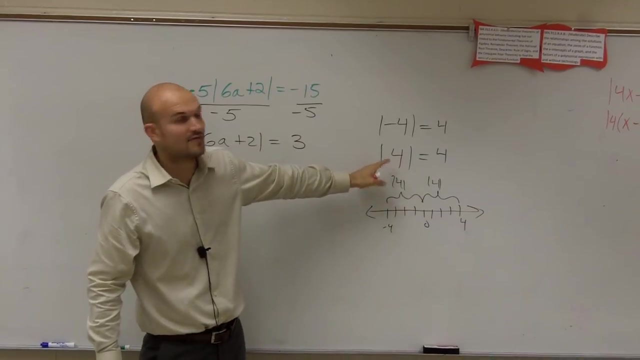 plus two is equal to three. Now remember for it to equal three we could have, inside of here it could be positive three, or inside of here could equal negative three. right, Because if it equaled positive three, if it equals positive three, then the positive version of an absolute. 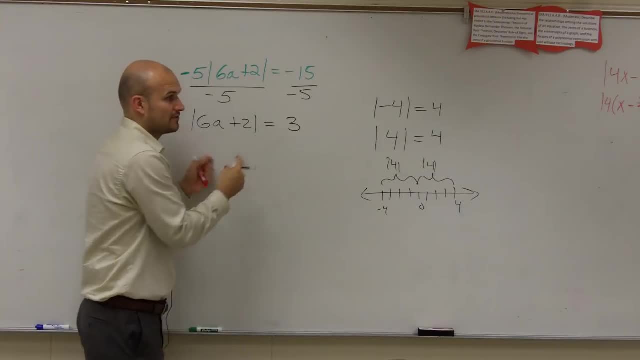 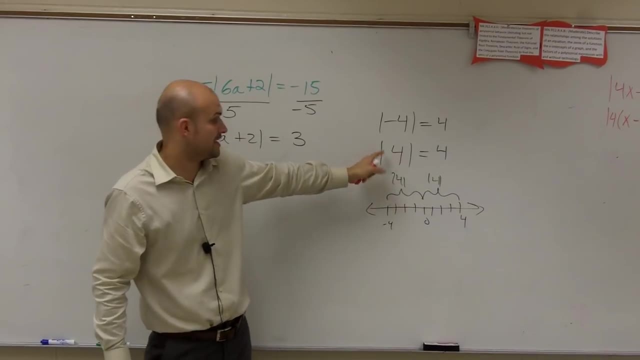 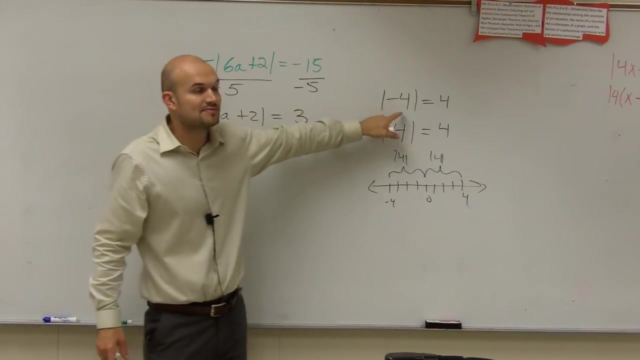 be positive 3, or inside of here could equal negative 3,. right, Because if it equals positive 3,, if it equals positive 3,, then the positive version of an absolute value equals negative 3.. And this inside here could also equal negative 3,, because if the negative value of an absolute 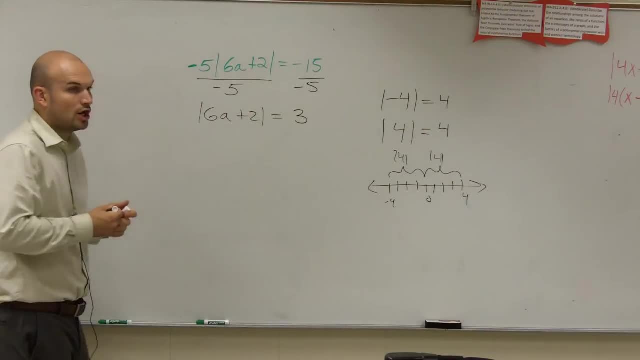 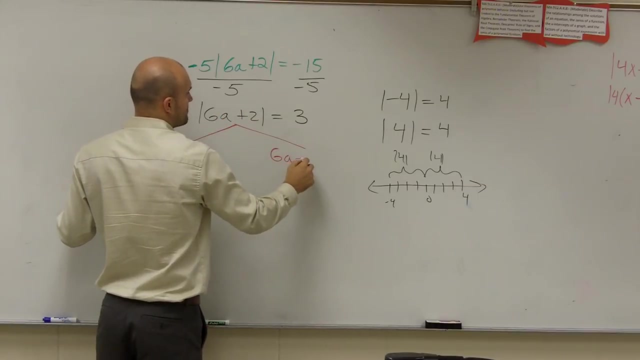 value also equals 3.. So what I'm going to do is what we call set up two cases. My first case is going to be: 6a plus 2 equals 3, meaning this inside of here can equal 3.. And then also 6a minus 2. 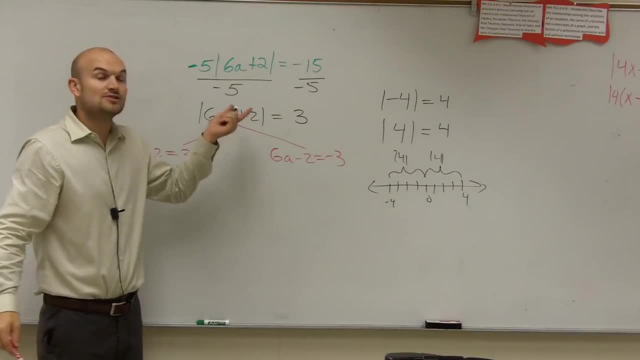 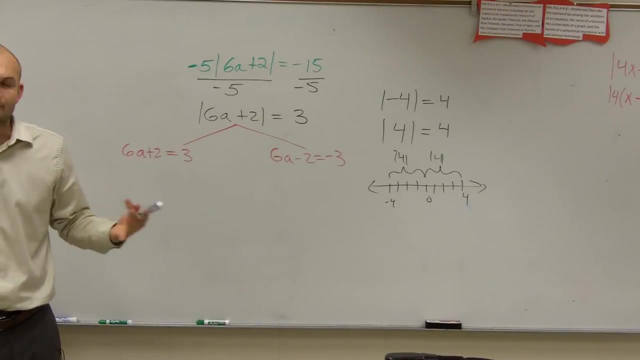 could also equal negative 3.. So, inside of here, could also equal negative 3,, because it doesn't matter If this equals 3 or negative 3,, my answer is always going to be 3 by the absolute value sign. So now, ladies and gentlemen, we have two-step equations, right? This ain't bad, We can solve. 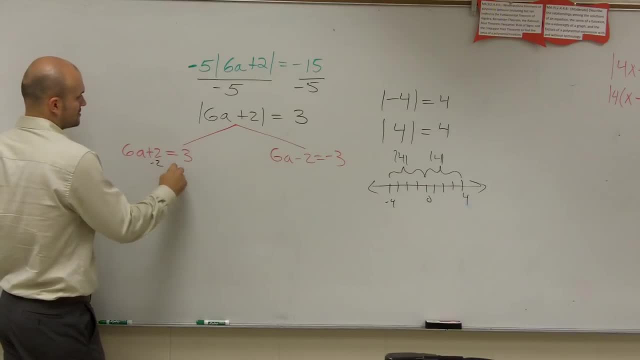 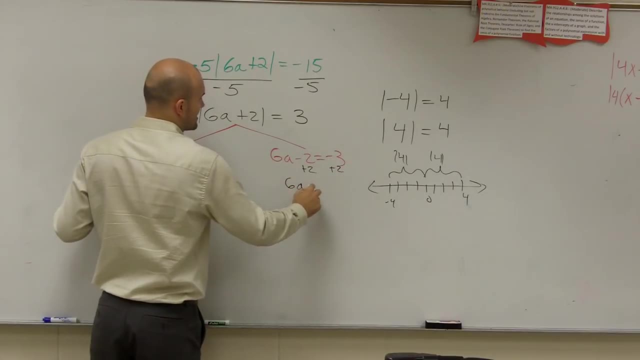 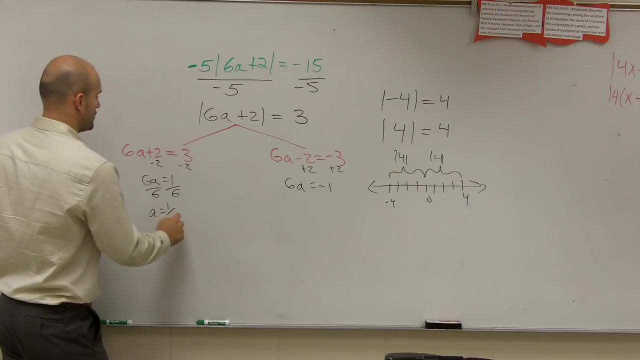 this stuff. So to solve here: subtract the 2, add the 2. So I get 6a equals 1. Here I get 6a equals negative: 1. Divide by 6.. a equals 1 over 6.. 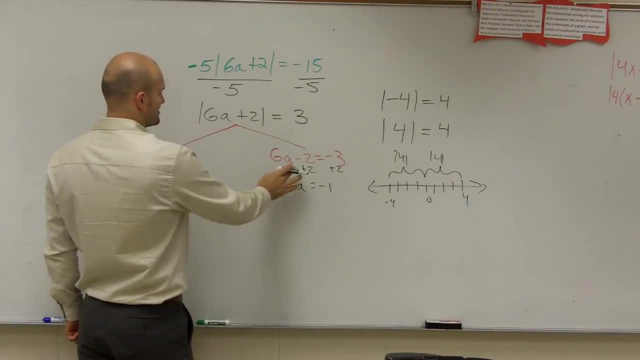 Here I divide. Why is it plus 2?? Yeah, I was going to say that's minus plus 2.. I was going to say that doesn't make sense. Minus 2, so I get negative 5.. Then I divide by 6. So I get a equals negative. 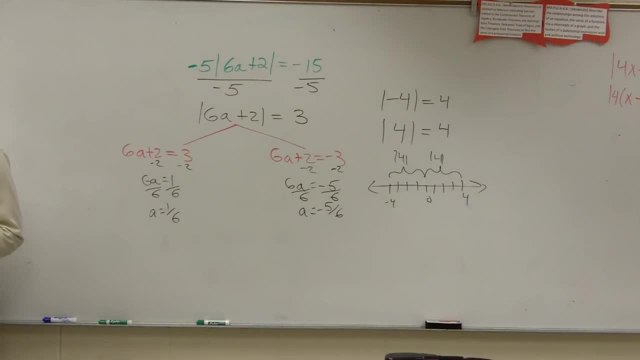 5 over 6.. Now the next thing that's important for us to understand about this is we need to make sure we check our solutions. So I'm going to write a nice check, And what I'm going to do is I'm going to plug in each one of these values in for a, So I write absolute. 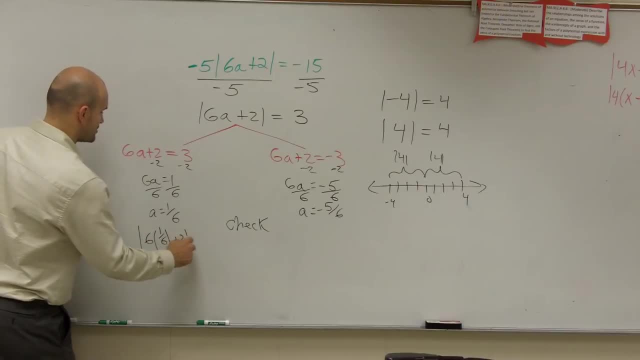 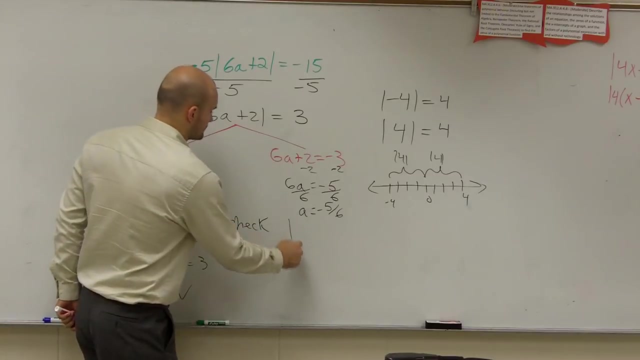 value of 6 times 1. sixth plus 2 equals 3.. 6 times 1, sixth is 1.. 1 plus 2 is 3.. Absolute value is equal to absolute value of 3.. Is that equal to 3? Yes, it is. Check Next one. Absolute value of 6. 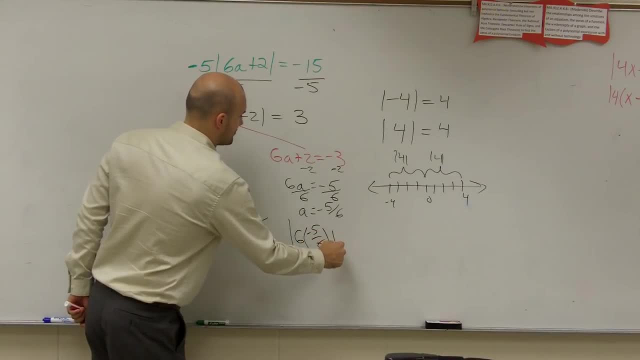 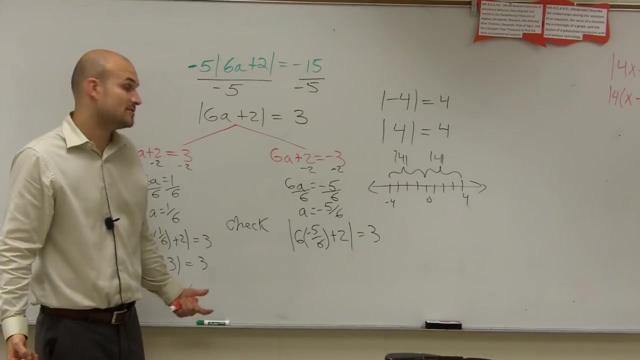 times negative: 5 over 6 plus 2.. 6 plus 2,, 6 plus 2 minus 2,. right there, Absolute value equals 3.. There we go. 6 times negative: 5 over 6. That's equal to negative 5.. Negative 5,. I'm sorry. 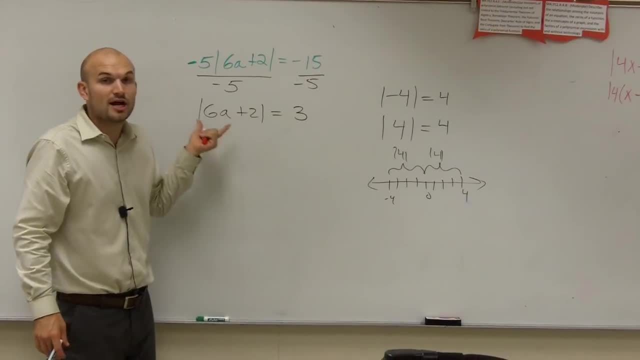 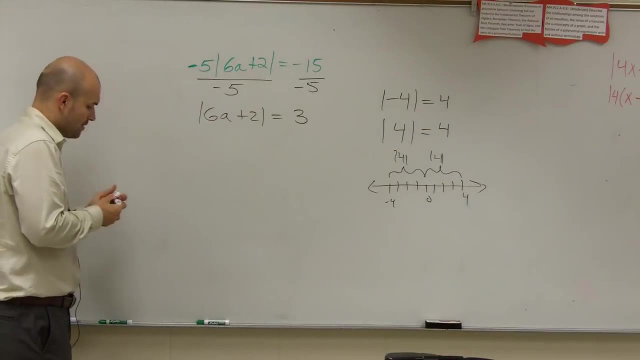 value equals the number, And this inside here could also equal negative three, because if the negative value of an absolute value also equals three. So what I'm going to do is what we call: set up two cases. My first case is going to be: 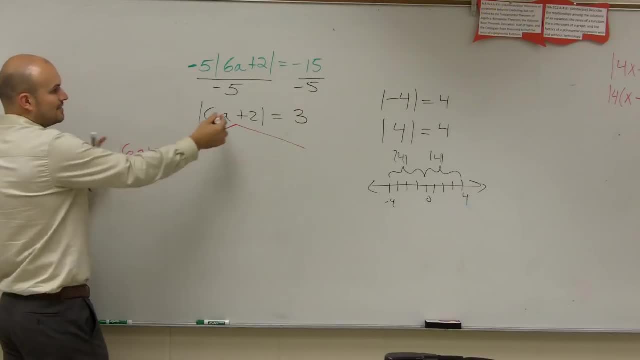 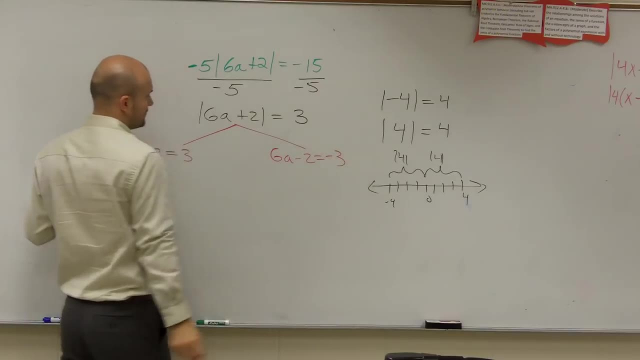 six a plus two equals three, seeing meaning this inside of here can equal three. And then also six a minus two could also equal negative three. So inside of here could also equal negative three, because it doesn't matter if this equals three or negative three. 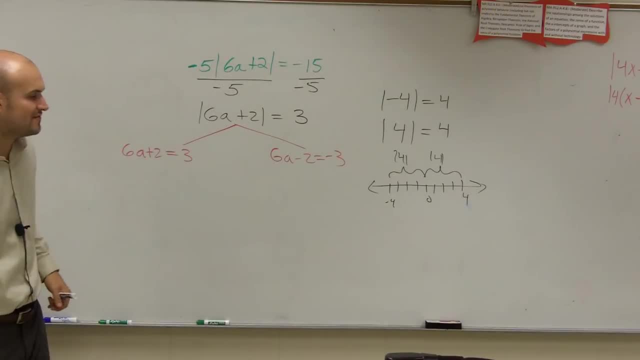 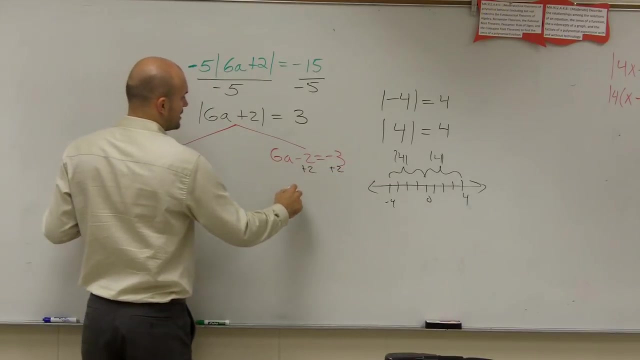 my answer is always going to be three by the absolute value sign. So now, ladies and gentlemen, we have two step equations, right, This ain't bad, We can solve this stuff. So to solve here, subtract the two, add the two, So I get six a equals one Here, I get six a equals negative one. 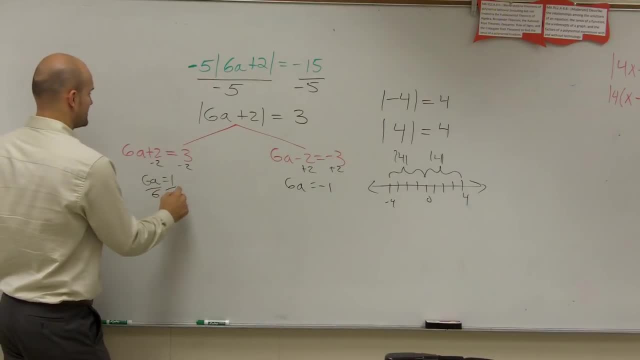 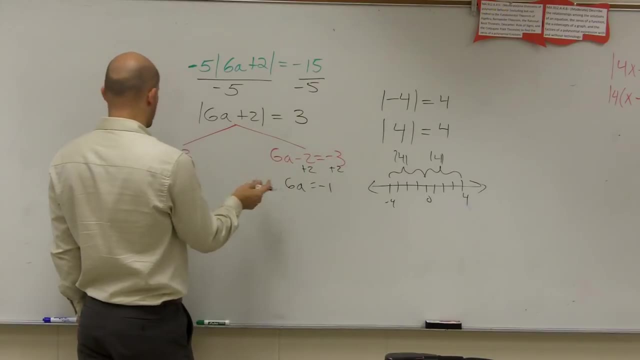 divide by six, a equals one over six. Here I divide by six, by two. I'm going to add a plus two. Why is it plus two? Yeah, I was going to say that's minus plus two. I was going to say that doesn't make sense. Minus two. so I get. 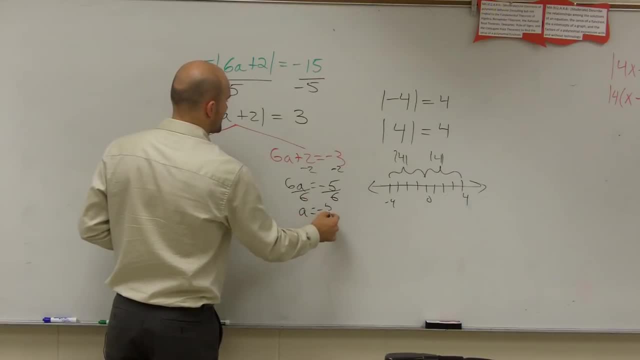 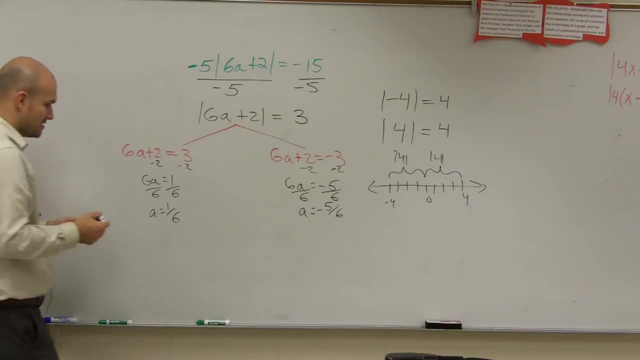 negative five, Then I divide by six, So I get a equals negative five over six. Now the next thing that's important for us to understand about this is we need to make sure we check our solutions. So I'm going to write a nice check, And what I'm going to do is 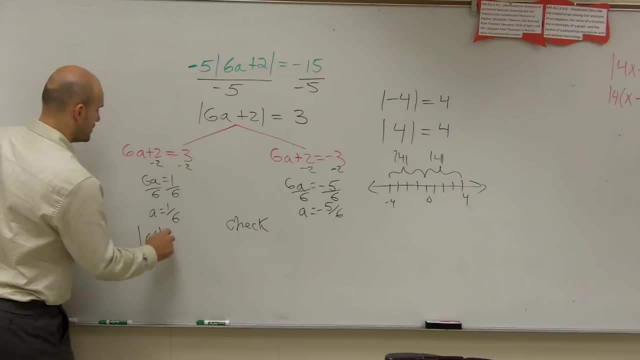 I'm going to plug in each one of these values in for a. So I write: absolute value of six. Sixth plus two equals three. Six times one-sixth is one. One plus two is three. Absolute value is equal to absolute value of three. is that equal to three? 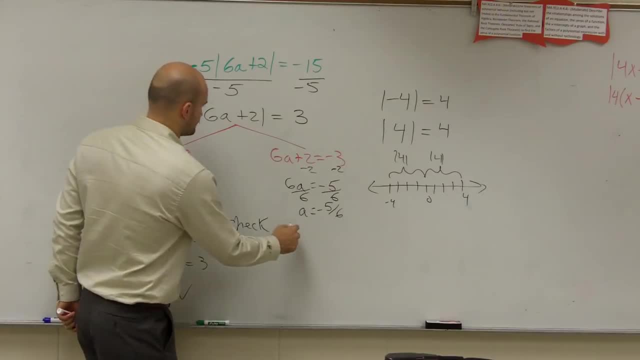 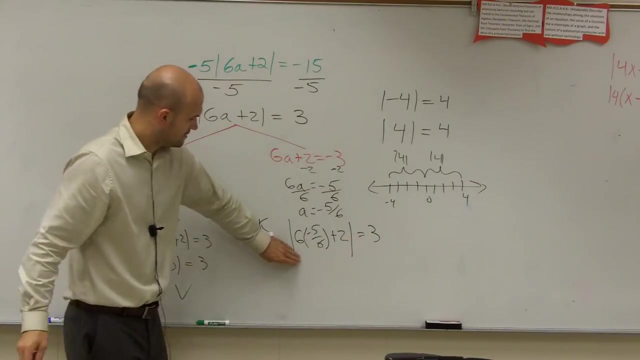 Yes, it is. Check Next one: Absolute value of six times negative five over six plus two. Six plus two, six plus two minus two: right there, Absolute value equals three. There we go. Six times negative five over six, that's equal to negative five. 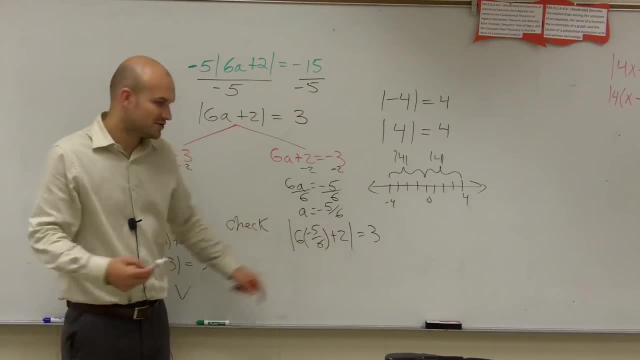 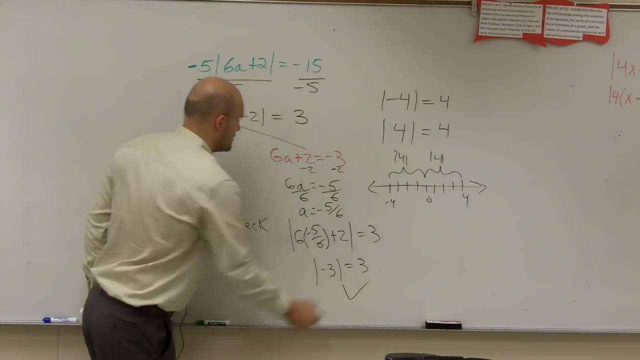 Negative five- I'm sorry, Negative five plus two is equal to absolute value of negative three, which is equal to three. Is that true or false? That's true. So there you go. Both solutions work. So, ladies and gentlemen, just to recap, whenever you're solving absolute value signs, 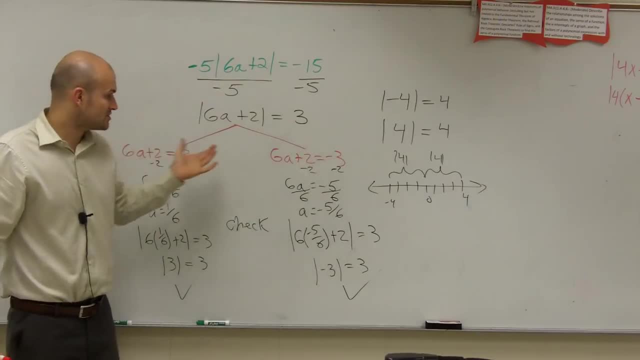 make sure you first isolate the absolute value, then solve for two separate cases, then check your work And there you go, That's it, That's it. 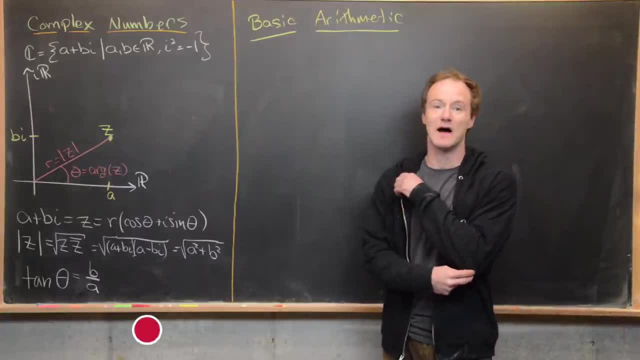 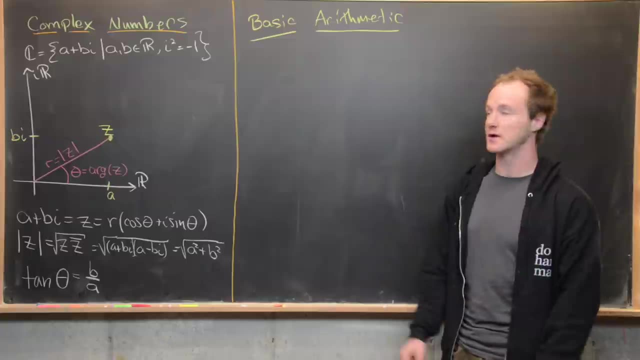 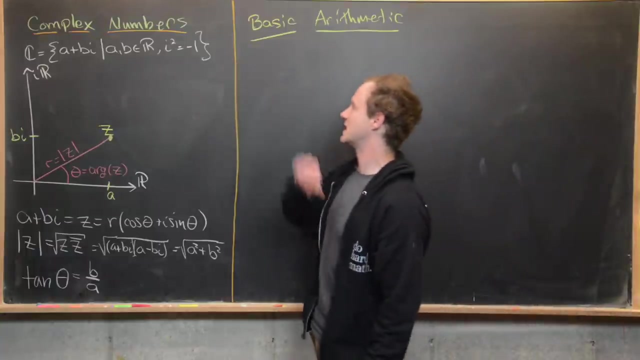 Here we're going to look at the basic tool of complex numbers as it applies to math problem-solving type problems, like from contests. But before we do that let's recall some really important and basic definitions. So the first: what is the set of complex numbers in the first place? So we'll take the set of complex. 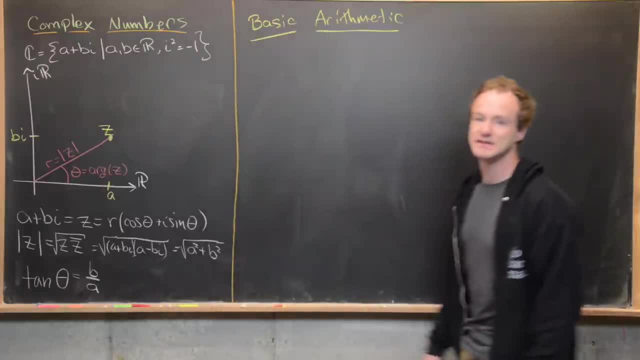 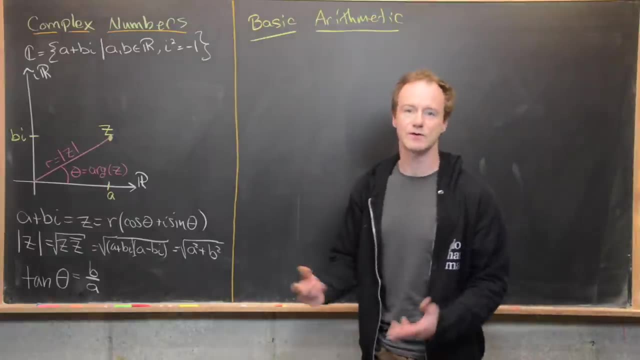 numbers to be all numbers of the form a plus bi, where a and b are both real numbers and i squared is negative 1.. So in other words, i is the square root of negative 1.. Okay, and then we can graphically express a complex number in: 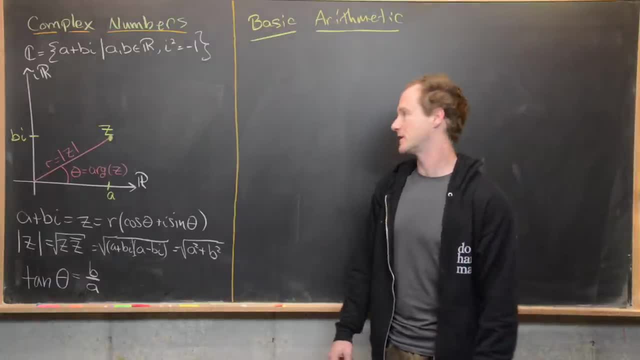 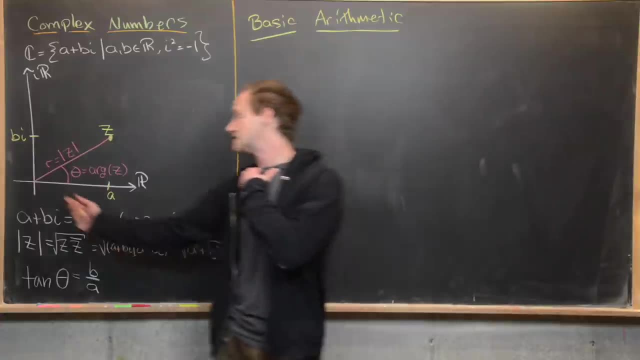 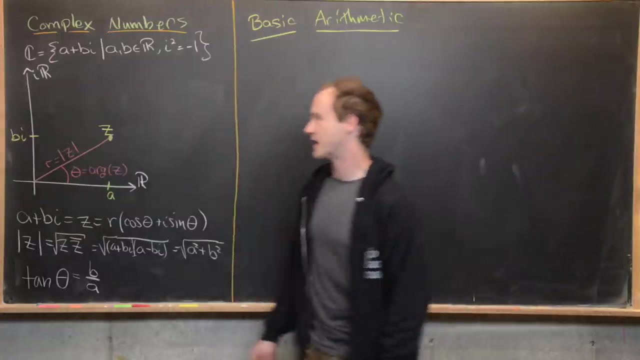 the following way. So it naturally lives in something called the complex plane, which has a real axis, which we generally put horizontally, and then it has an imaginary axis, which we generally make the vertical axis. So notice, I've got a real axis here and an imaginary axis there. That's i times r. 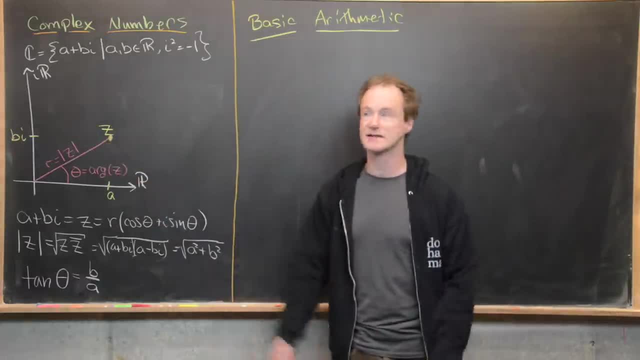 So we're going to have a real axis here and an imaginary axis there. That's i times r. So we're going to have a real axis here and an imaginary axis there. That's i times r. And then a number z, a complex number, I should say, which is equal to a plus bi. 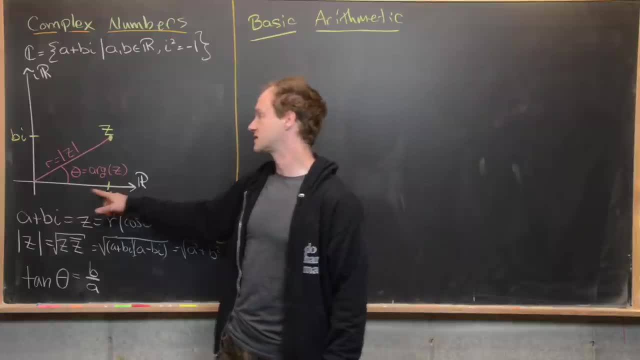 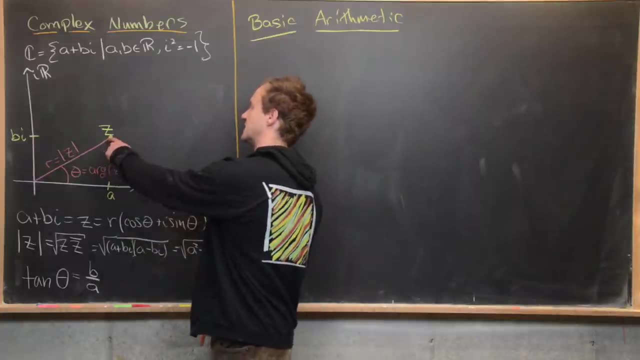 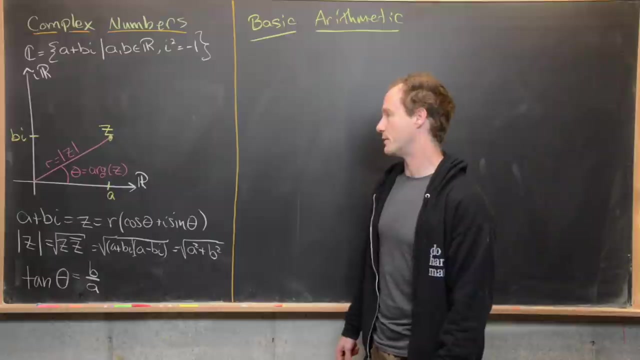 So notice we have gone a along the real axis and then b units along the imaginary axis. So that means this point right here is bi. So that makes this point right here: z, which is a plus bi. So in the Cartesian coordinate plane this would be like a comma, b. Good, And then there are two main ways to.